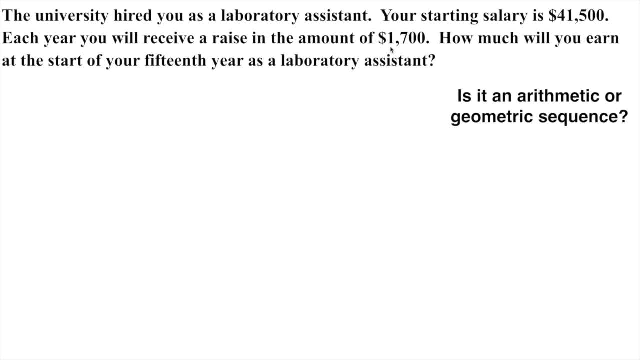 adding a certain number to it every time, And this one says you'll receive a raise in the amount of $1,700.. So it's a fixed amount. We're going to get the same amount every time. So that would be an arithmetic sequence. Now that we know, 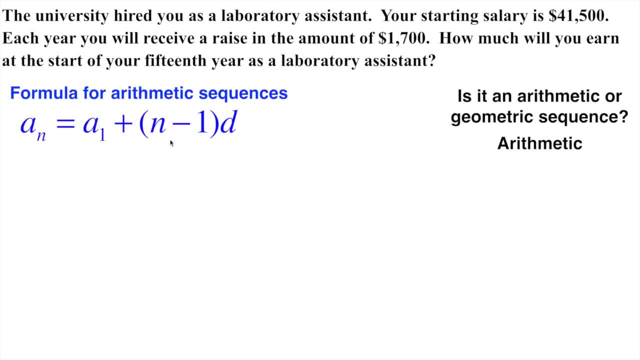 that we can bring in our formula for arithmetic sequences- And this is just kind of a generic formula for arithmetic sequences- And we start plugging in some information. So we're going to start plugging in some information. We're going to start plugging in some information that we know. We know what the starting. 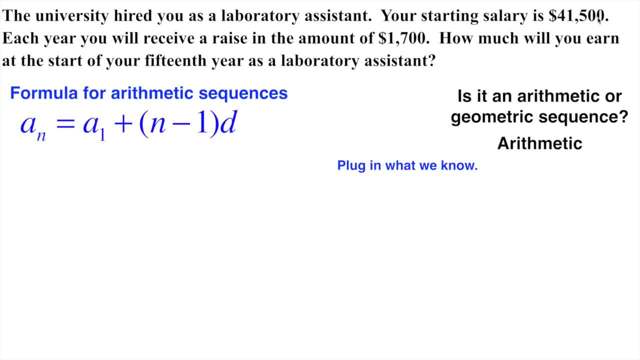 amount a of 1,. this is our first year. We're going to make $41,500.. We also know what the difference amount is going to be. It's a common difference. It's going to be $1,700.. We're going to make $1,700 more every single year that we work. 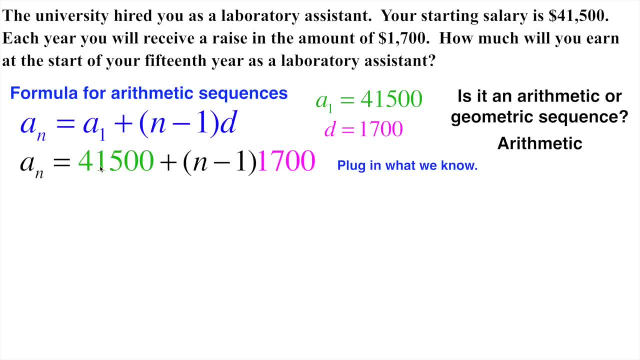 there. So now I kind of plug both of those in. Okay, this is my a of 1, my first. my starting amount $41,500.. $1,700 is how much I go up every single year. Now this one asks how much we will earn at the start of our 15th year. So 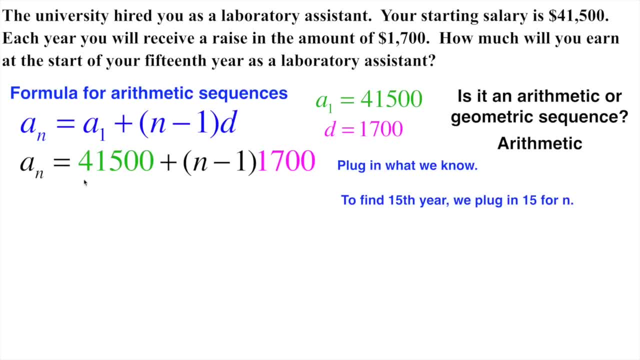 now what I'm going to do is plug in 15 for n. So right here and right here, I'm going to plug in 15.. So I've done that here. Now, to find out how much I'm going to make for the 15th year, all I need to do. 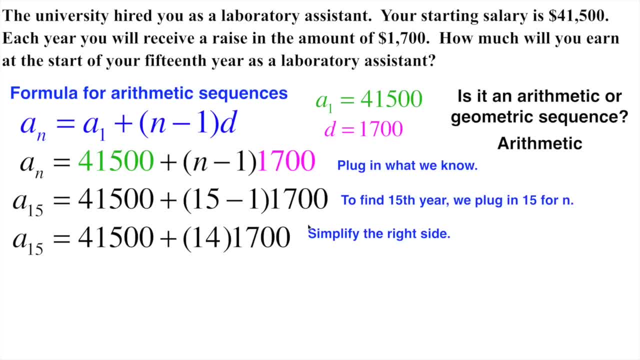 is: simplify what's on the right-hand side. So I go: 15 minus 1 is 14.. 14 times 1,700 is $23,800.. I add that to my initial amount of $41,500 and that gives me. $65,300.. Now you can put a dollar sign on there- commas, all those will be fine. When you're typing it into the online system, just write it at $65,300.. It'll be just fine, The computer. 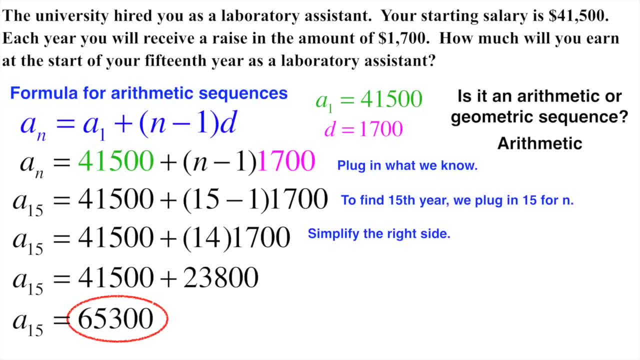 has a hard time when you try to put labels in it. So just leave it at $65,300 is fine, Or $65,300, I should say.